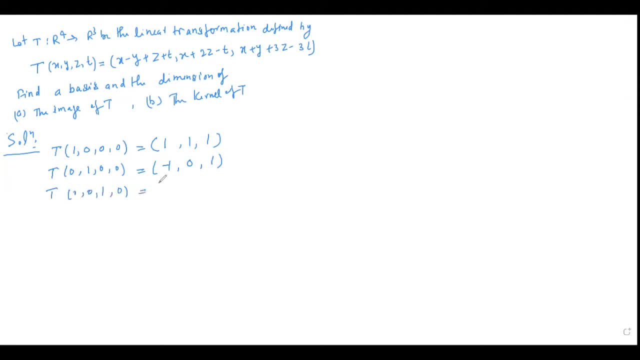 1 comma 0. We get 1 comma 2 comma 3.. Then again, put t is equal to 0 comma 0, comma zero comma one. we get one comma minus one comma minus three. so the image vectors expands image of t. hence they form a form of matrix and 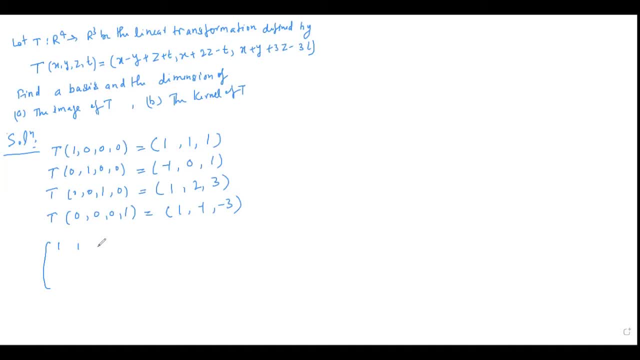 apply row reduce echelon form to reduce this matrix up to echelon form. so minus one: zero one. one two, three one minus one minus three. so we have to reduce this form to row: reduce echelon form. so first r1 mean first row will be same. there is no change in r1. 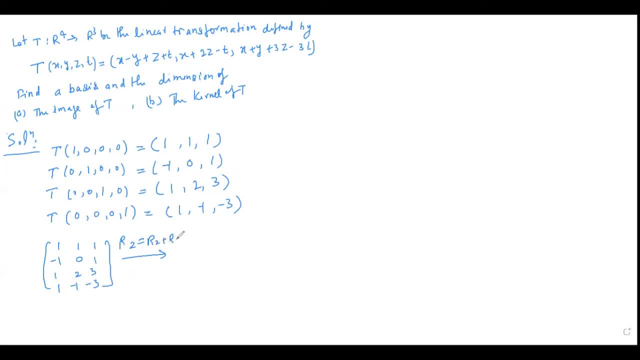 and r2 is equal to r2 plus r1, r3 is equal to r3 minus r1, and r4 is equal to r4 minus r. so what we get: first row is same one, one, one, and then zero. one plus zero is one, one plus one is two. then, uh, third row minus first row, so one minus one is zero. 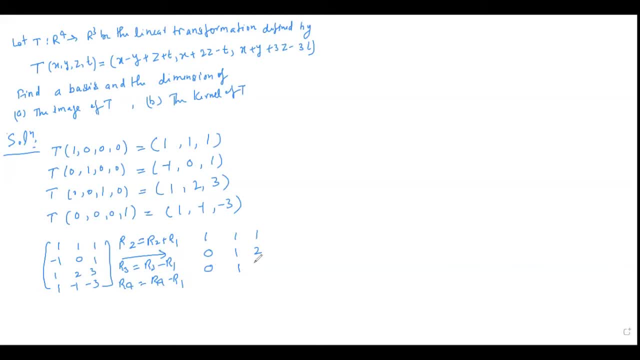 two minus one is one, three minus one is two, and then again r4 minus r1, so one minus one is 1 is 0, minus 1 minus 1 is minus 2, minus 3 and minus 1 is minus 4.. 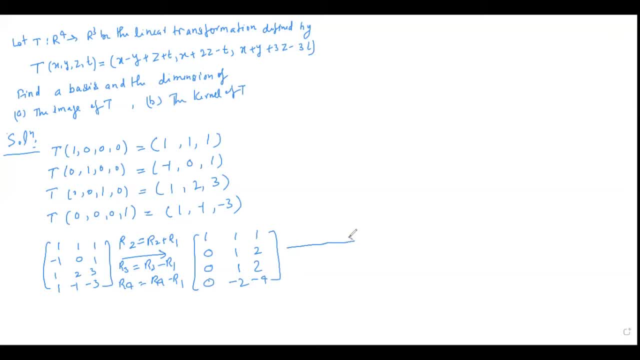 Now first two row will be same, third and fourth. there is a change in third and fourth, so for third row, R3 is equal to R3 minus R2 and R4 is equal to R4 minus 2 R2, R4 plus. 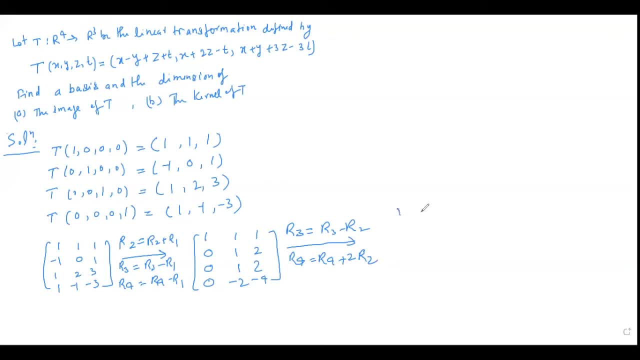 2 R2.. So what we get? 1, 1, 1, 0, 1, 2, then 0, 0, 0, 0, 0 and 0.. So here we have two independent rows: 1, 1, 1, 1, comma, 1, comma 1 and 0, 1, 2, and they 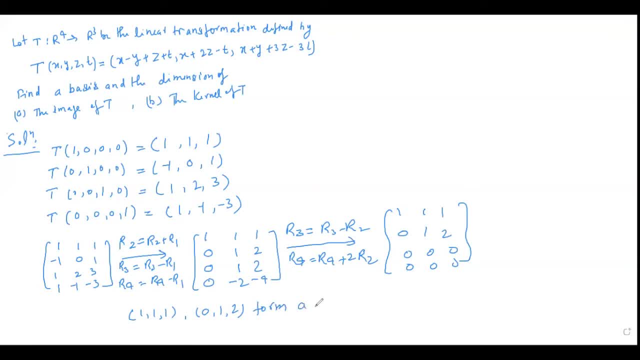 form a basis. They form a basis for image. So here we have two independent rows, 1, 1, 1, 1, comma, 1, comma 1 and 0, 1, 2, and they form a basis. 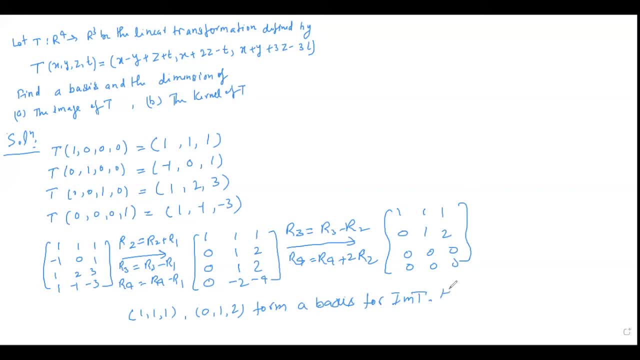 So we have two independent rows, 1, 1, 1, 1, 1, comma, 1, 0.. Hence, difference in dimension: we have given r, followed by H ik riq equals 13.. Now, we are going to, We are going to. 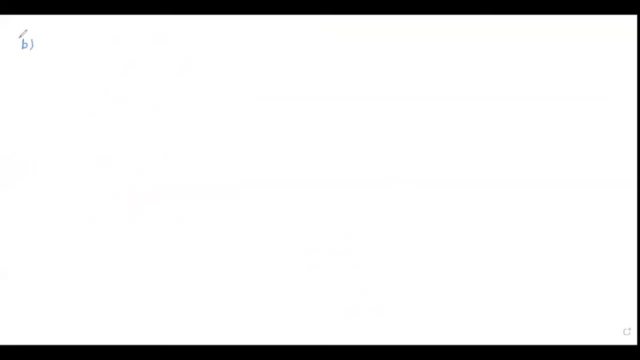 214.. 1, 2 is the extension of T. Hence Dimension of image is equal to T. for second part, we know that t of V is equal to zero. it is come now Right. So here V is equal to X. be play. 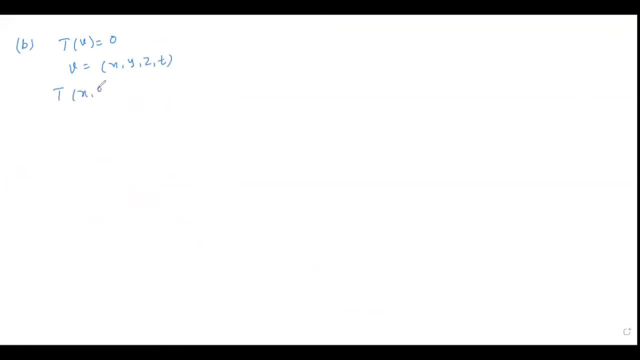 why they come as E come up To the middle of X commaima, to the middle Television of sugar t. So t of x, y, z, t is equal to 0.. So what is the definition of this? x minus y plus z plus t? 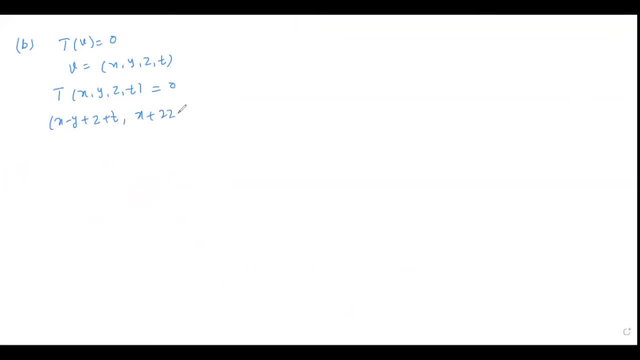 comma x plus 2z minus t. comma x plus y plus 3z minus 3t is equal to 0. 0 means 0 vector of 3. So this is 3.. So from there we have three equations: x minus y plus z plus t is. 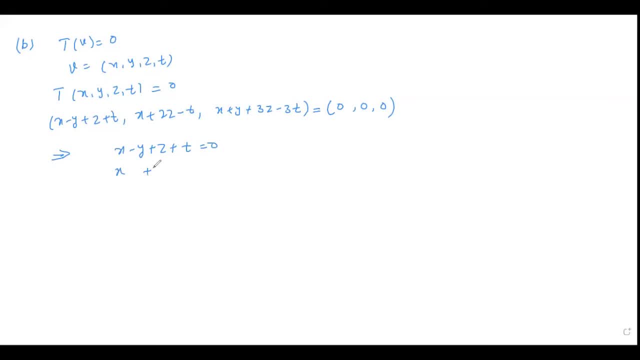 equal to 0.. x, 2z plus 2z minus t is equal to 0, and x plus y plus 3z minus 3t is equal to 0. Now again form a matrix. This is for a 3 by 4.. 1 minus 1, 1, 1.. 1, 0, 2, minus 1, 1, 1, 3,. 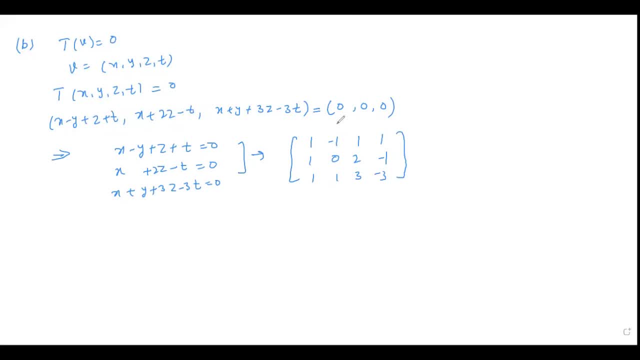 minus 3.. So first row would be same. Reduce it up to the row reduced equivalent form. So R2 is equal to R2 minus R1 and R3 is equal to R3 minus R1.. So 1 minus 1, 1 and 1.. So 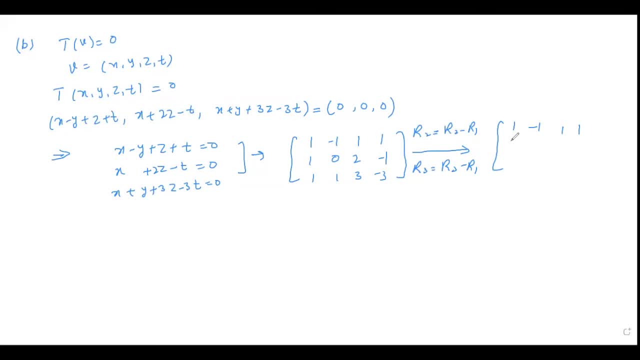 R2 is equal to R2 minus 1.. Means 1 minus 1 is 0.. 0 plus 1 is 1.. 2 minus 1 is 1.. And minus 1 minus 1 is minus 2.. Again, 1 minus 1 is. 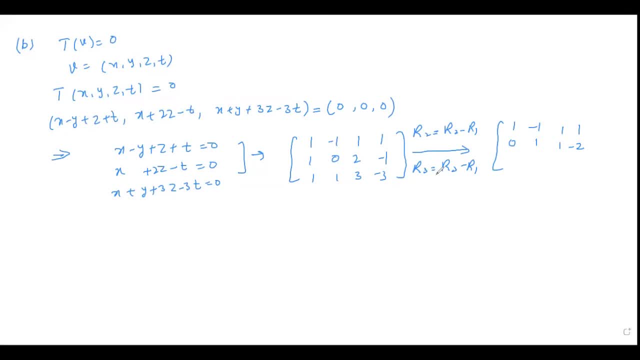 0. Means R3 is equal to R3 minus 1.. R3 minus R1.. So 1 minus 1 is 0.. Then 1 minus minus plus means 2.. Or 3 minus 1 is 2.. And minus 3 minus 1 is 2.. So 1 minus 1 is 0. And minus. 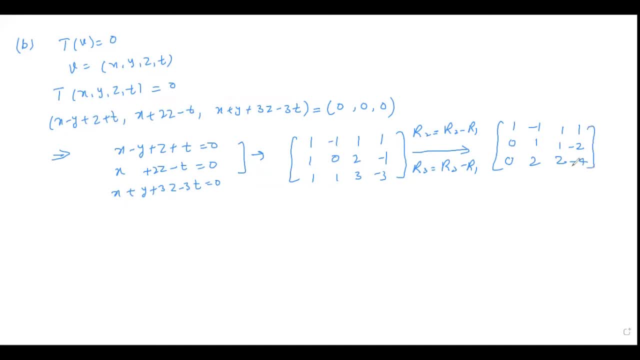 4 is minus 4.. So R3 is equal to R3 minus 2, R2.. We get 1 minus 1, 1, 1, 0, 1, 1, minus 2 and 0.. 2 minus 2 is 0.. 2 minus 2 is 0.. Minus 4 plus 4 is 0. So R3 is equal to R3 minus. 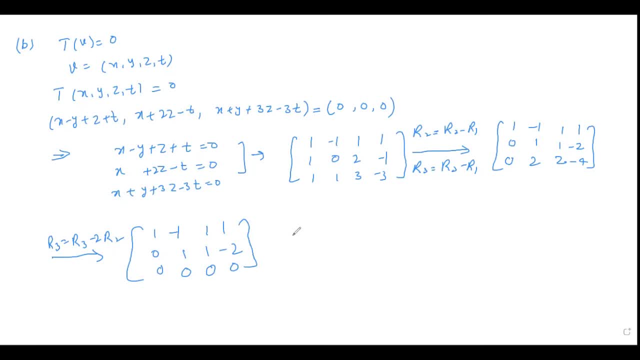 0.. So from this matrix we have two equations in the form of x, y, z and t. So first one is: x minus y plus z plus t is equal to 0. And second one is y plus z minus 2t is equal. 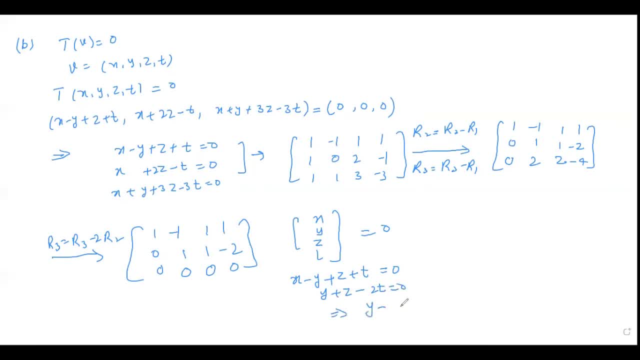 to 0. So from this equation, y is equal to 2t plus z minus 2t is equal to 0. So from this equation, y is equal to 2t plus z minus 2t is equal to 0. So from this book we: 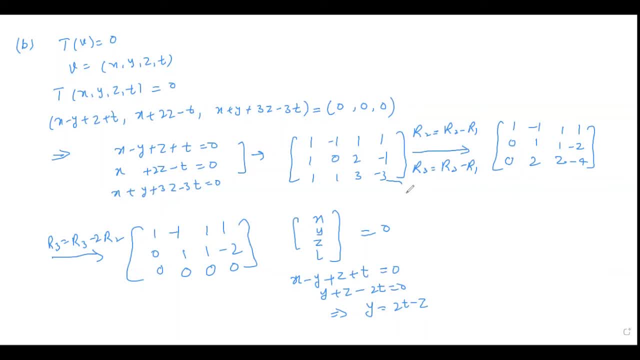 have written that x minus 7 equal to 1 plus minus 2t minus z plus t is equal to 0.. And this expression, 1 plus 0 is equal to 0. So the first one is z minus 7.. Here, 2 variables are free: t and z. 2 variables are free, Hence dimension. 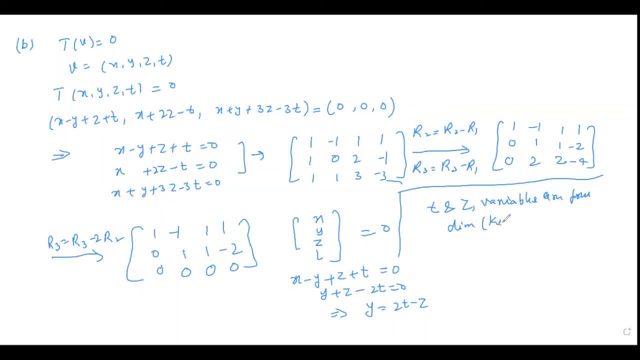 of kernel t is equal to 0. So that is the first version of this feature. Suppose z is equal to k1 and t is equal to k2. Then y is equal to 2k2 minus k1 and x is equal. 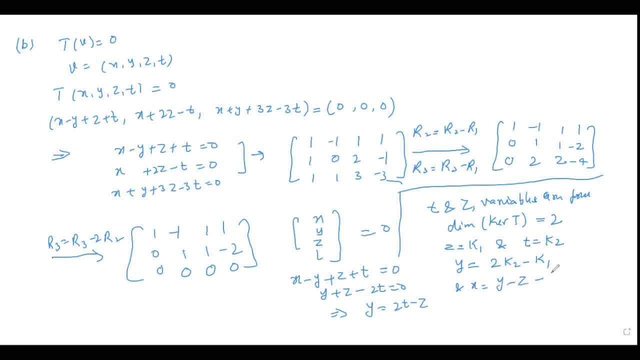 to y minus z minus t, So this is 2k2 minus k1, z is k1 and t is k2.. So from here we have k2 minus 2k. So write x, y, z and t And this is equal to. 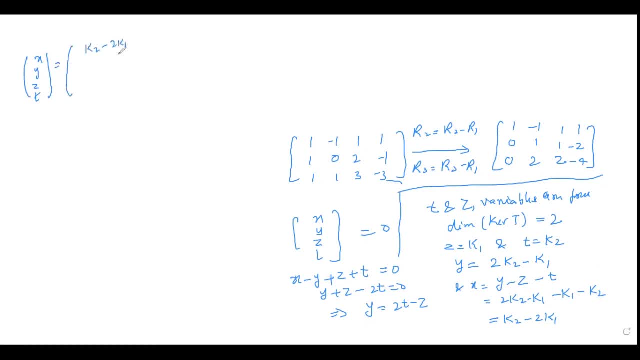 k2 minus 2k. So from here we have x, y, z and t. So from here we have x, y, z and k2 minus 2k1.. Then y is 2k2 minus k1.. Then z is k1 and t is k2.. So from here we may. 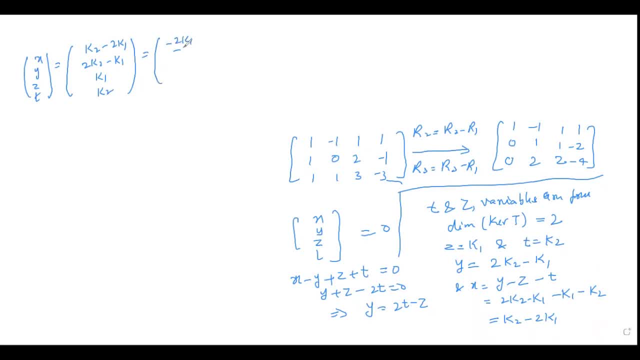 write minus 2k1 minus k1, k1 and 0 plus 2k2 minus 2k2 minus k1. So from here we have k2 minus 2k2 minus t and k2.. We have separated both of them. Now take k1, common from this. 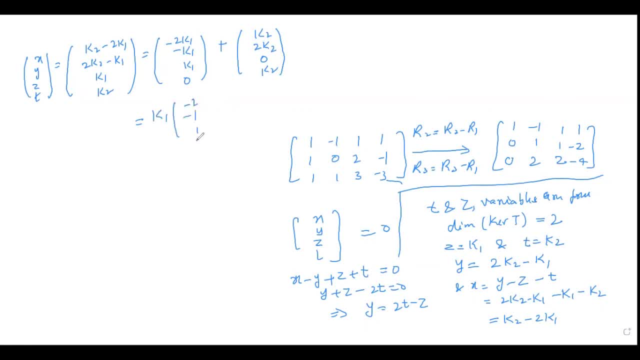 So we have minus 2, minus 1, 1 and 0.. And take k2 common from this one, So 1, 2, 0 and 1.. Hence minus 2, minus 1, 1 comma 0 and 1, 2, 0, comma 1 form basis. of kernel of T.